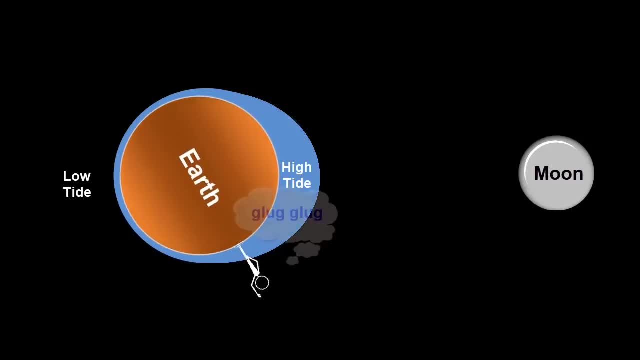 And a low tide where the oceans don't bulge. So you'd expect one high tide each day. But here it gets interesting, because there are two high tides a day. How come This? is because the strength of gravity is greater when objects are closer. 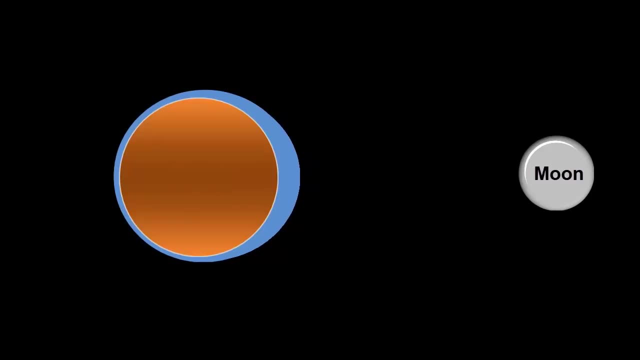 We'll call the location of the ocean on the near side of the moon point A, At the centre of the Earth, point B, And at the far side, ocean point C. The strength of the moon's gravity is strongest at A because it's closest to the moon. 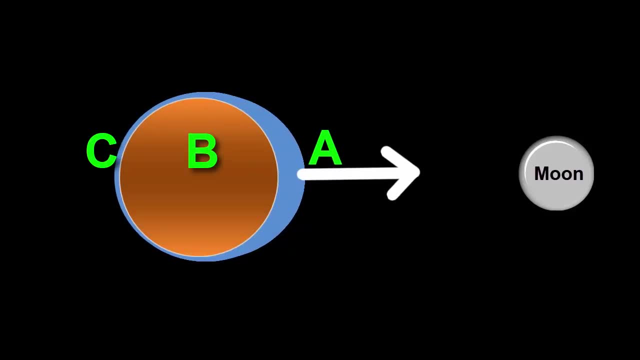 So the part of the ocean that bulges towards the moon most is at A, But the moon's gravity also pulls on the Earth, moving it towards the moon as well. This has two effects. First, it makes another bulge at C. 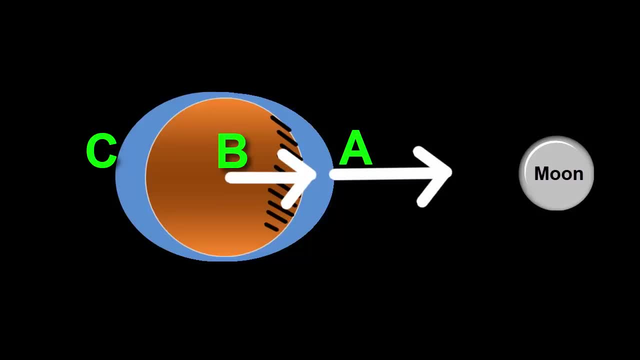 Second, it fills in the air. Second, it fills in the bulge at A, But not completely, because A has moved further towards the moon than B. Lastly, the far side ocean at C is also attracted to the moon, But it moves least because the moon's gravitational pull here is at its weakest, being farthest from the moon. 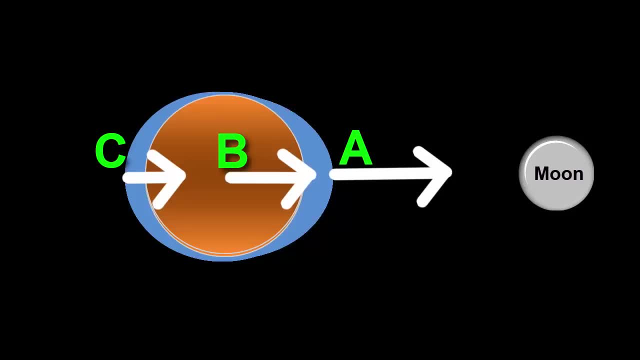 This leaves a partial bulge at C, though not as big as the one at A. Now we can see why, when the Earth rotates through 24 hours, it goes through two high tides and two low tides. But there's another surprise. 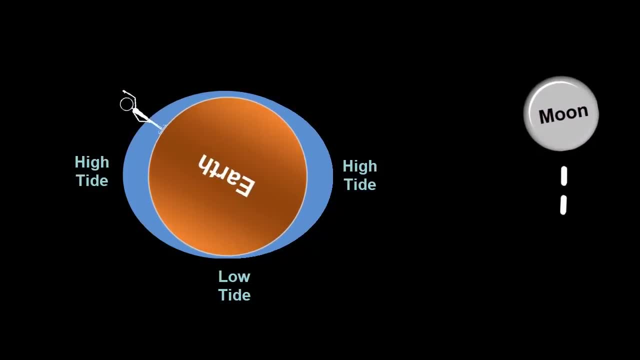 By the time, the Earth has rotated once and arrived back at its original position. the moon has moved on a bit because it's orbiting the Earth at the same time. That means that the moon has moved a bit. That means that the moon has moved on a bit because it's orbiting the Earth at the same time.